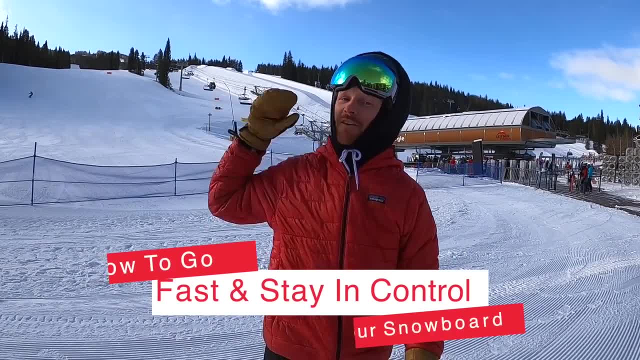 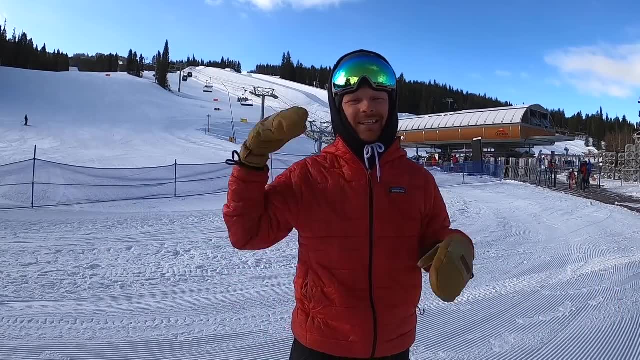 What's up guys? Tommy Bennett, here and today I'm gonna teach you how to go fast on your snowboard, But, more importantly, I'm gonna teach you how to stay in control while you're doing it. So make sure you stay tuned and stick to the end. if I miss anything, you got something to add. 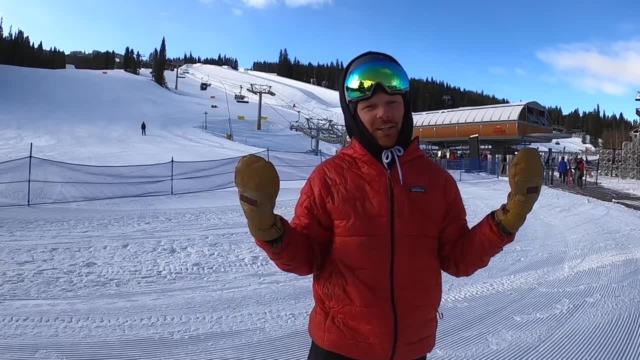 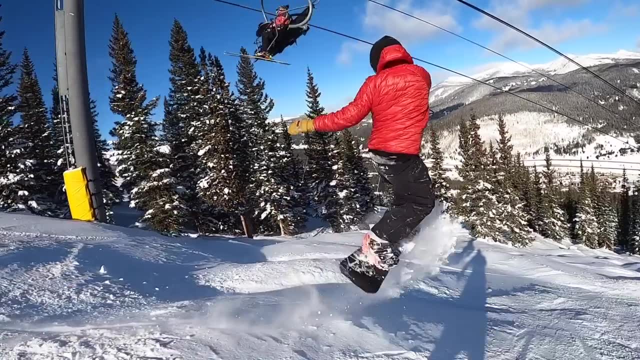 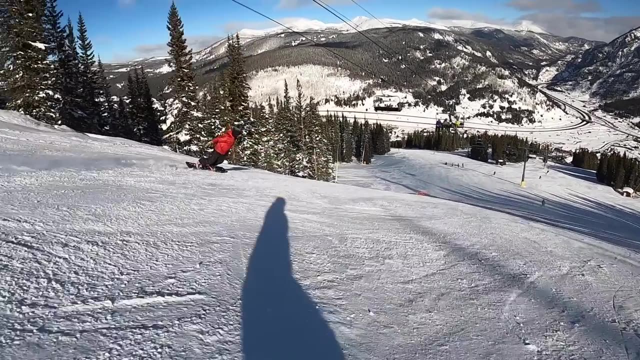 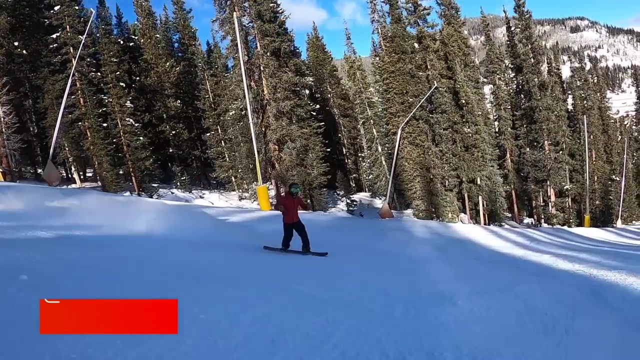 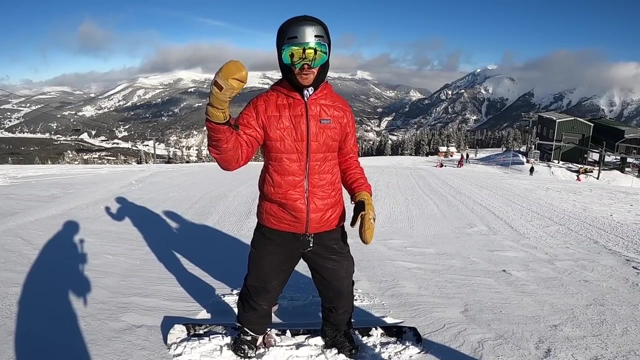 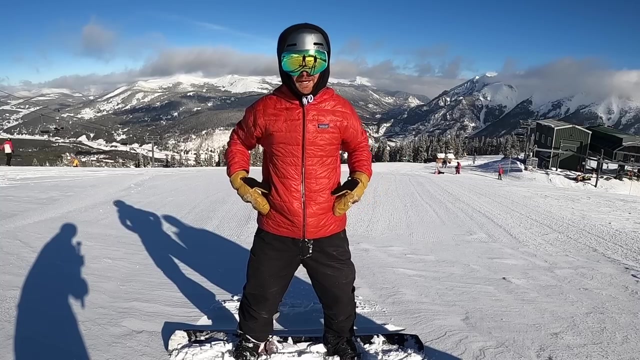 Make sure you put in the comments below: Awesome guys, Let's get started. So when it comes to going fast, You got to be in a body position that allows you to either put on the brakes or be stable. So what I want you guys to do is have your shoulders, your hips and your knees all stacked on top of each other. 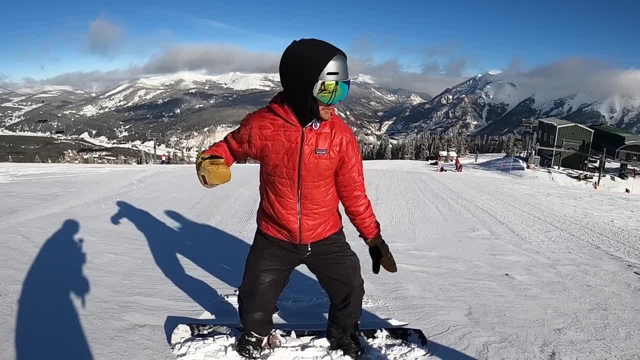 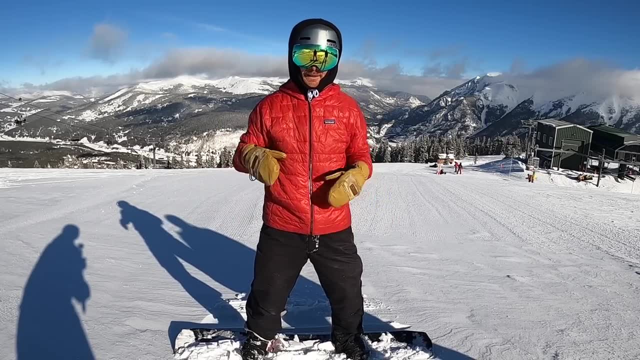 And then when I'm going this direction, I'm in this strong position. Imagine you're like weightlifting: you have a bunch of weight on your back. if I'm here, It's a very weak position. in addition, if my lead shoulders super open, How much time does it take to get on my toe side edge? 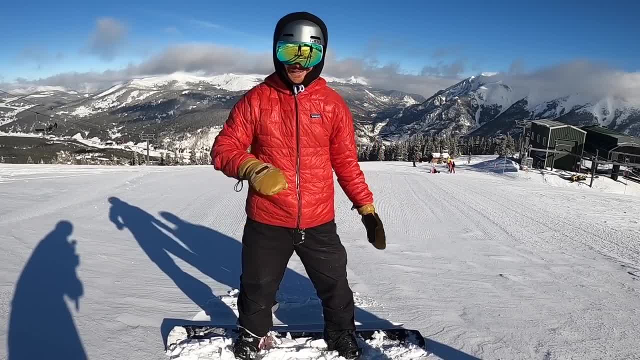 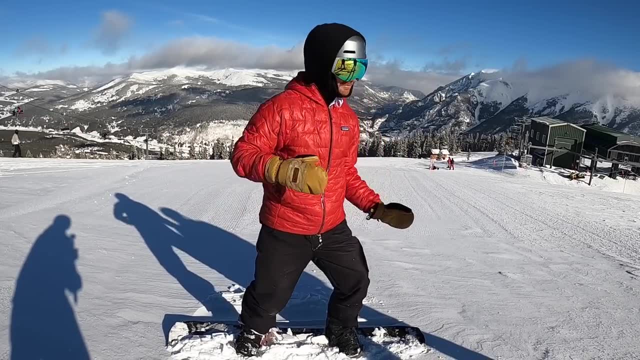 I have to go back to Center and then apply weight- not as ideal, But if I'm already in this position, in the center, in a neutral position, It's really easy to go to my toes, to my heels. This movement is gonna be super fast. Now it's gonna be key when we're going fast, because you're gonna have to be able to get on that toe side edge. 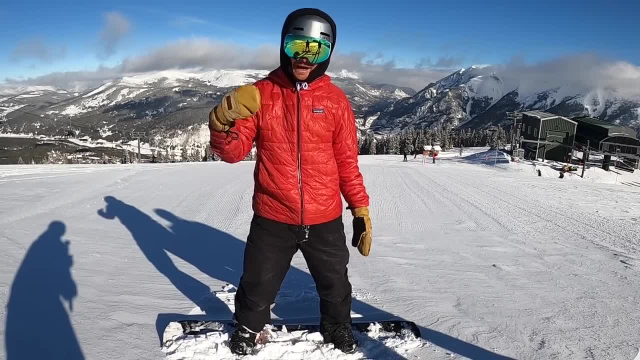 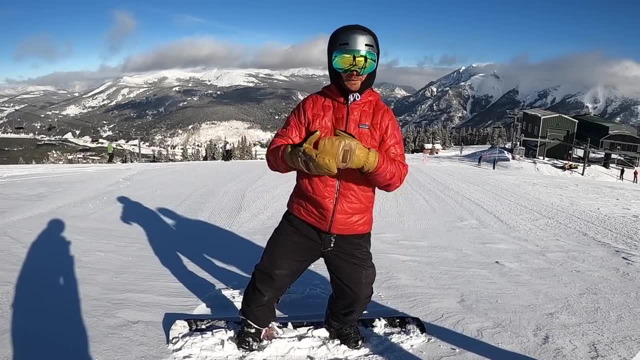 Intentionally, and then your heel side intentionally. now, after that, if you take your belly button and sink it down, You're gonna be in a strong athletic position. you know the same position we've learned about in high school. We're in this lower body position. 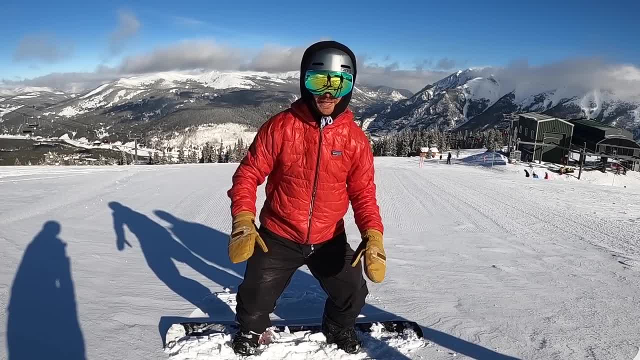 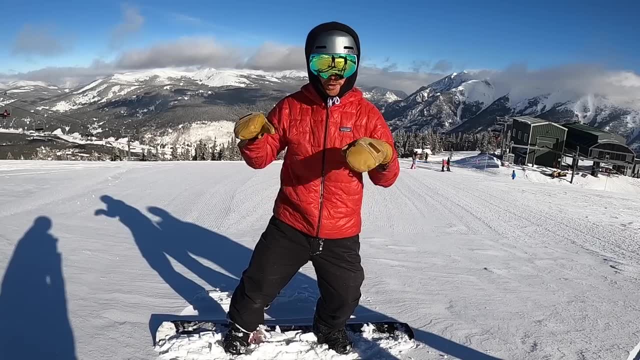 We're gonna be able to absorb the terrain or push away with our knees. that allows us to stay in contact With the ground the whole time, and that's gonna be key too. The more you're in contact with the ground, the easier it is to turn your snowboard if you're just bobbling like this. 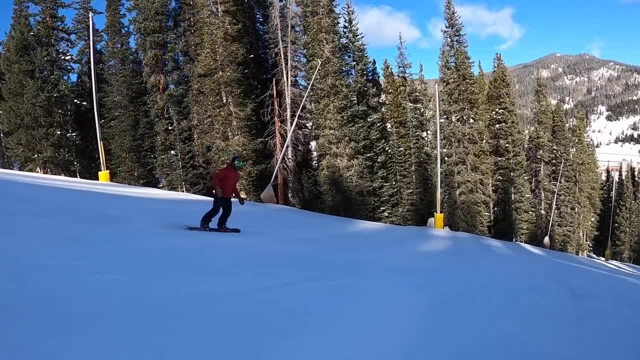 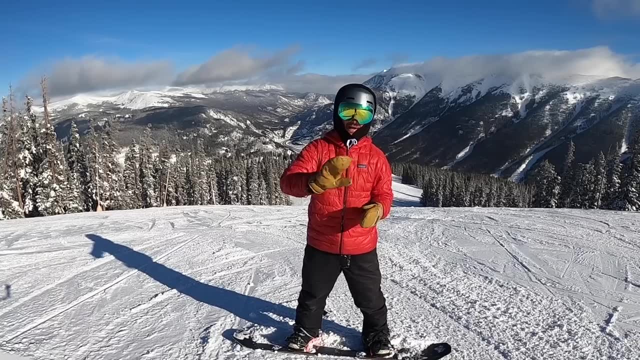 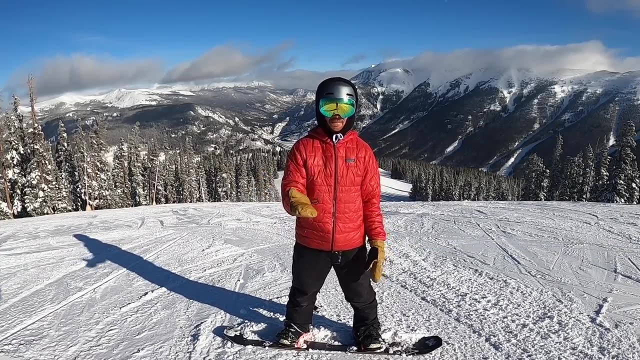 not sick. When it comes to going fast, the number one thing is being able to stay in control, But, more importantly, you got to be able to stop. So I'm gonna explain stopping on our heel side to heel side really quick now when we're doing a heel side turn. 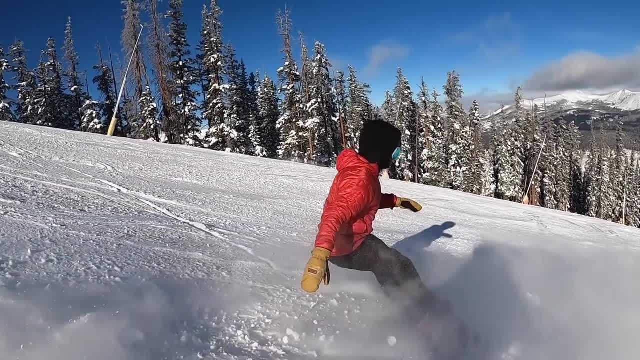 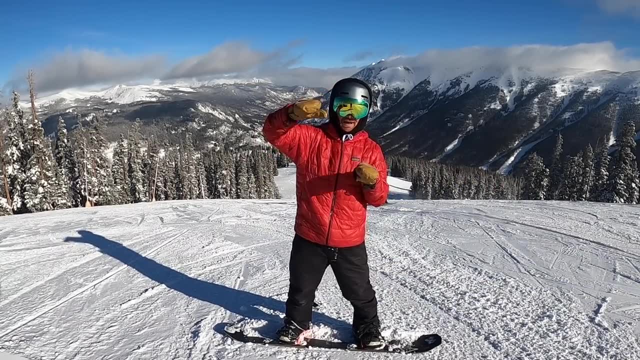 You want to make sure your belly button is as stacked over the edge as possible. Well, I'm gonna show you a clip of me exaggerating a hillside stop, And if my belly button and my center of mass goes too far down, I'm gonna end up slipping out. 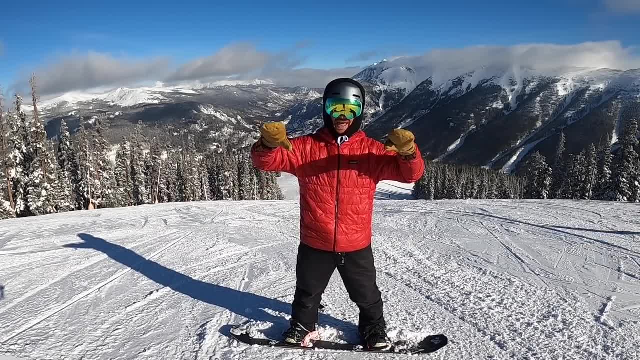 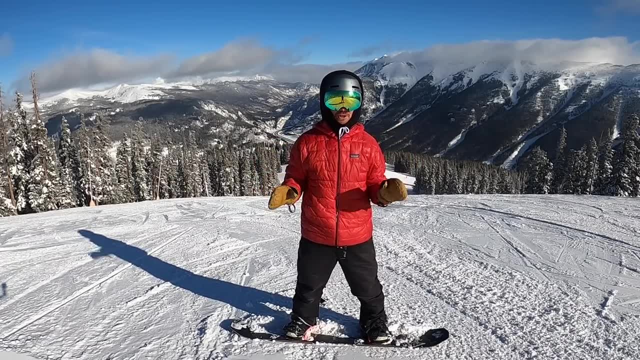 the other thing that will happen is if you put too much of an aggressive edge angle and you're tilting too much, your board is Gonna start skipping and then, just as I talked about earlier, if your board is not in contact with the snow, You're not gonna be slowing down. 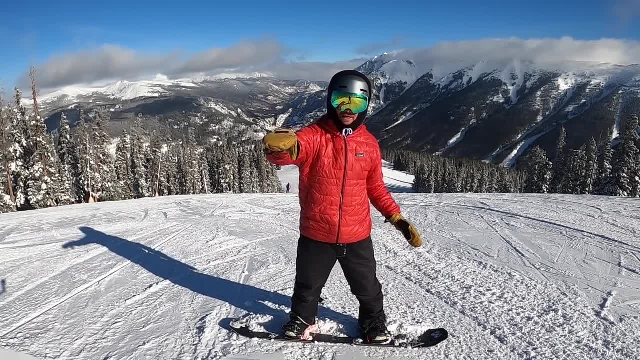 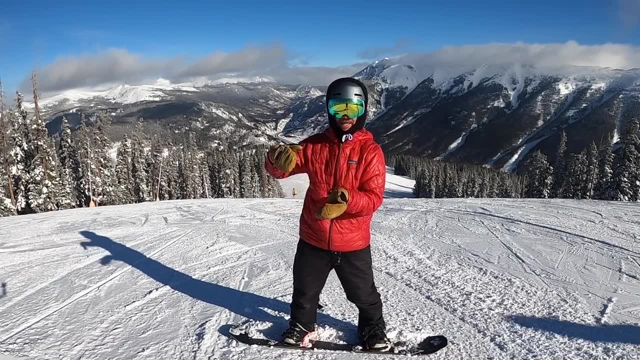 So what we're gonna do now is I'm gonna point the board straight down the hill and then I'm gonna try to stop as soon As possible. now, this is an exercise you can do on its own, an isolated movement. go fast, slow down. How fast? 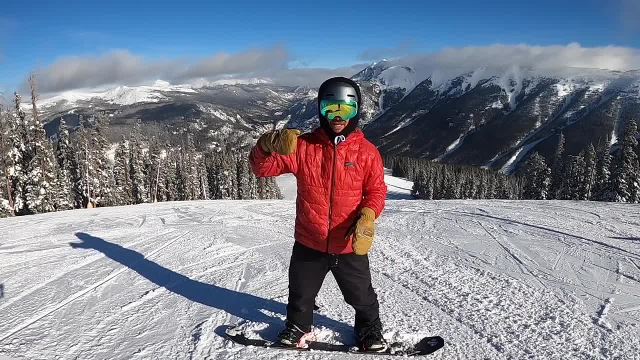 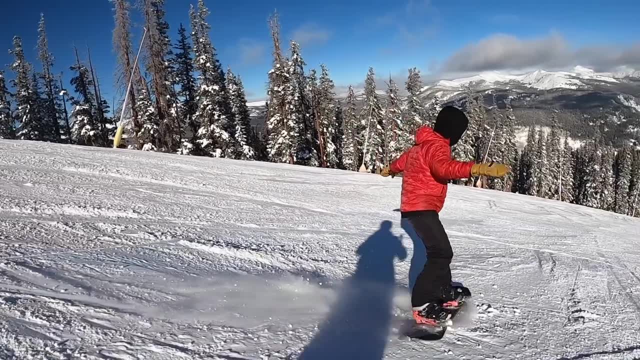 Can you slow down? this actually could be a really cool competition you do with your friends: go fast, Who can stop the fastest while staying in control? That's gonna be very important to going fast is knowing you can stop. That's also important to being on aout stand up. 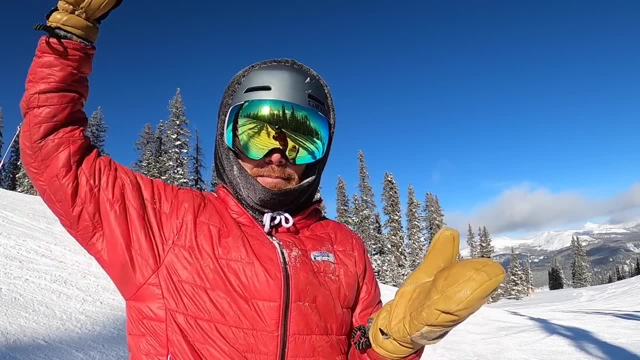 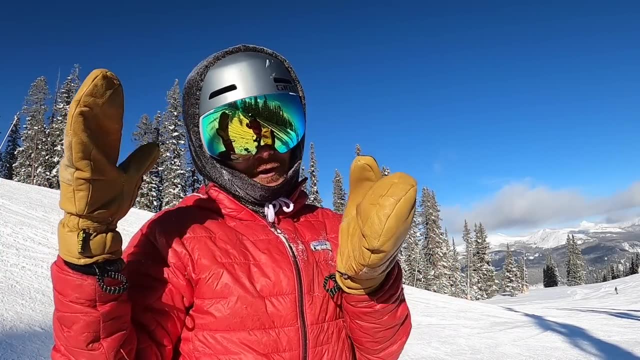 So within that exercise you'll notice that I am being able to slam on the brakes. I'm getting my belly button close to the board, So I'm in a strong, compact position, but I'm not leaning over too far now. if I lean over too far, I'm gonna end up. 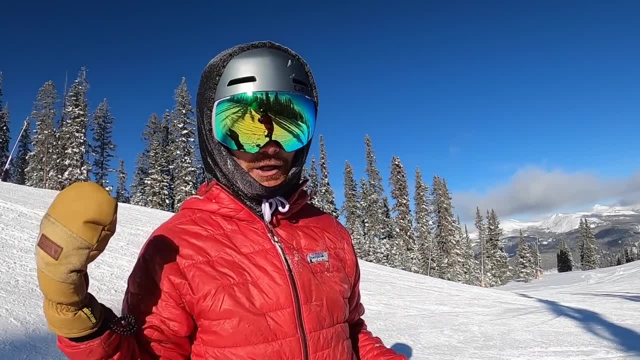 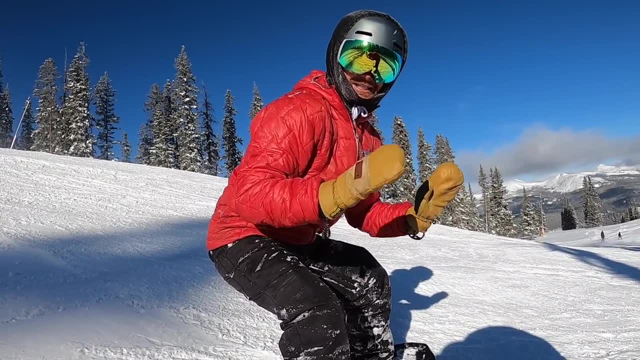 slipping and sliding and then end up like falling on my butt, as you just saw there. so it's important that you get your belly button low, that you're lifting up your toes and you're in a strong position like this so you can handle the braking position. but as soon as my belly goes back here, I'm falling. 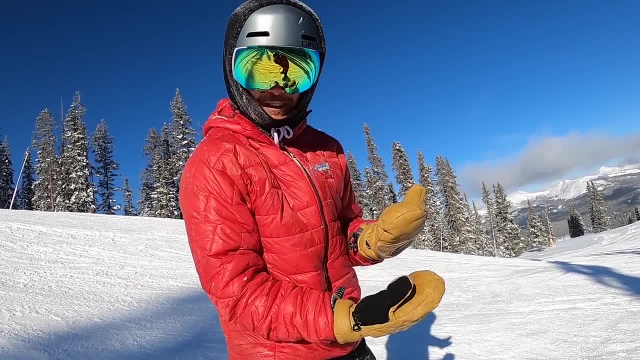 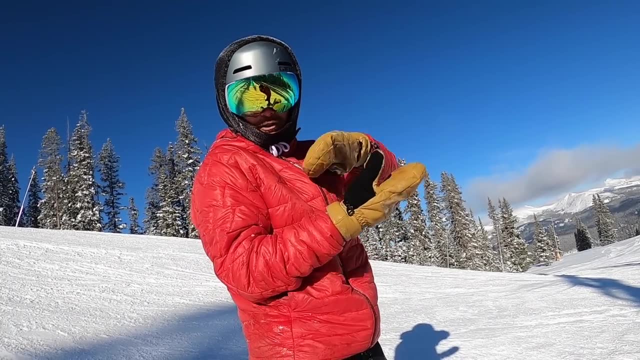 over. so now the same thing is gonna apply when it comes to our toes tight edge. we want to make sure that our belly button is getting low. now we're leaning over that. we're in a strong, athletic, balanced position. but if we go too far we're gonna chatter, we're gonna slip out, we're not gonna be able to stop. so 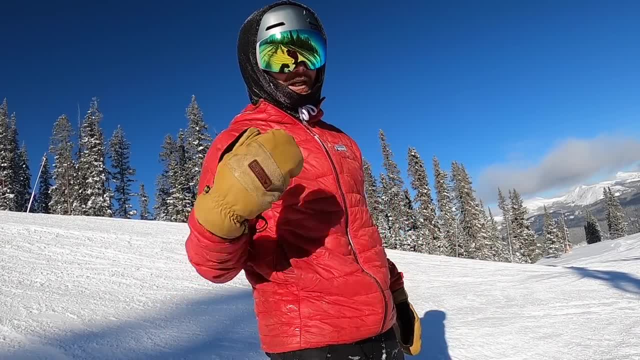 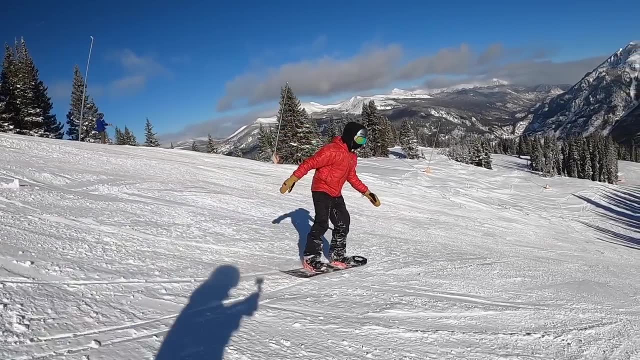 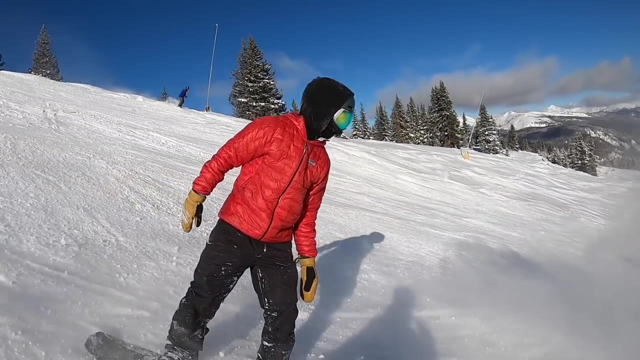 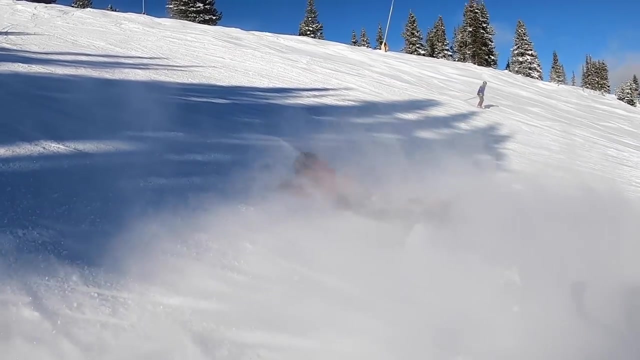 that's kind of counterproductive. I'm gonna show you a couple toe side edges, a couple toe side turns and braking, and now we're gonna start cooking it. all right, you guys ready? so when it comes to going fast, obviously I want you to stay in control. now there's 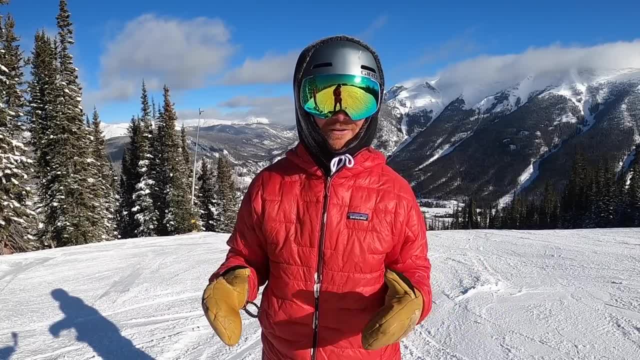 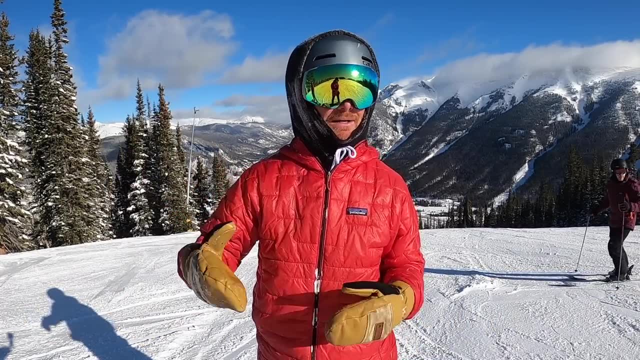 a couple things to consider: make sure that you're not cutting anybody off, you're not getting super close to anybody, and then you're choosing appropriate terrain. now, a lot of the times, your blues and blacks are gonna be a lot steeper, with less restrictions when it comes to speed. also, there are 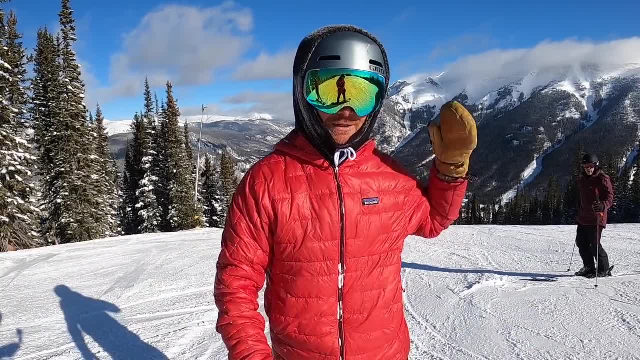 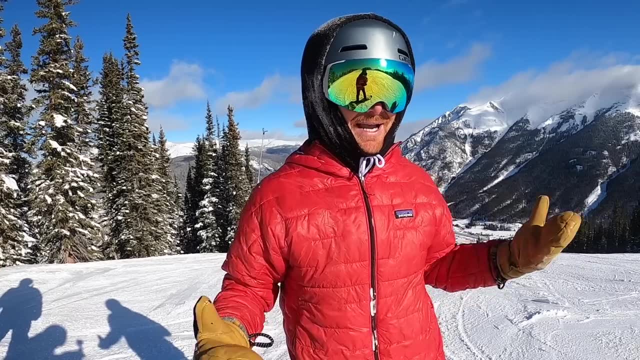 some resorts that allow no straight lining. straight line essentially means you're going flat base and absolutely no turns, so make sure that your body by the rules and you know what's going on. alright, guys? so now we're gonna get into some steeper terrain, so we're gonna have Jonathan Buckhouse here. he's gonna. 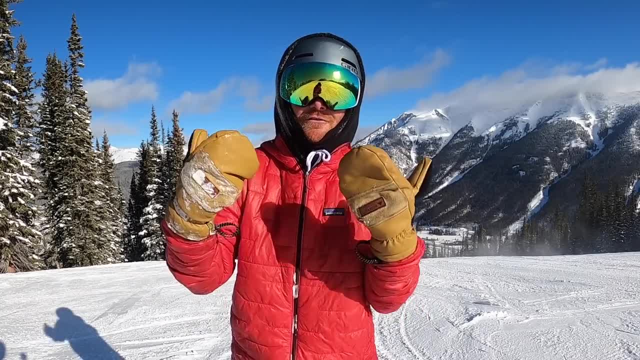 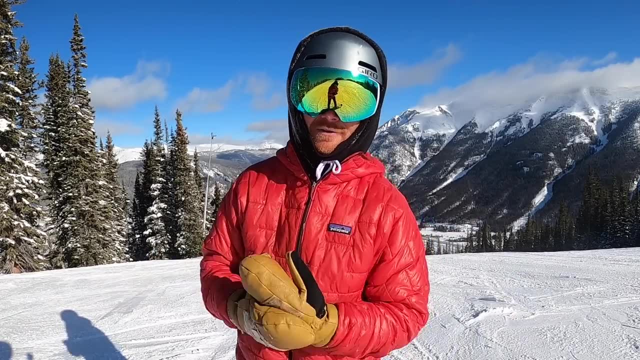 follow me on some of this steeper terrain so that you guys can get a feel and a sight of what I'm doing. when it comes to my turns again, make sure you're looking around, make sure you're not getting taken out or cutting anybody off. so, Buckhouse, you ready, my dude? oh, I'm ready, dude. 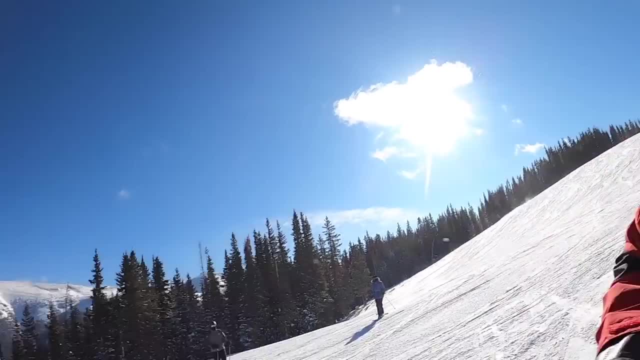 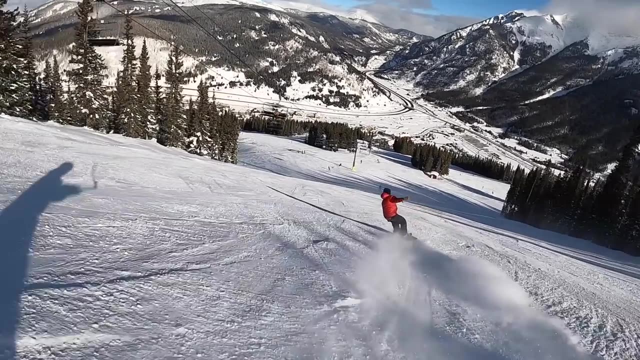 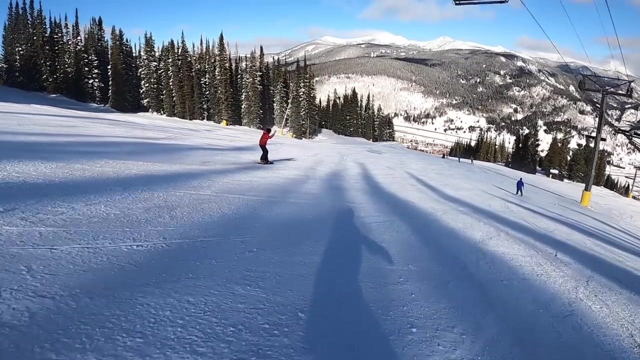 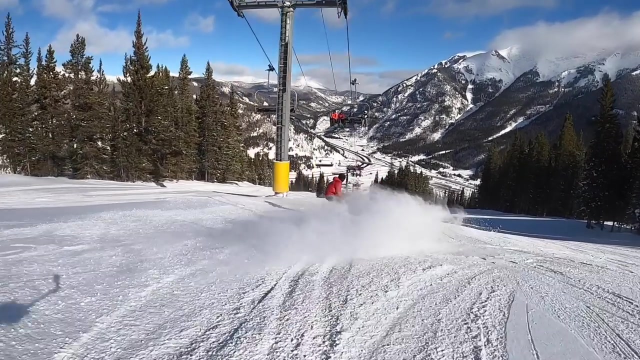 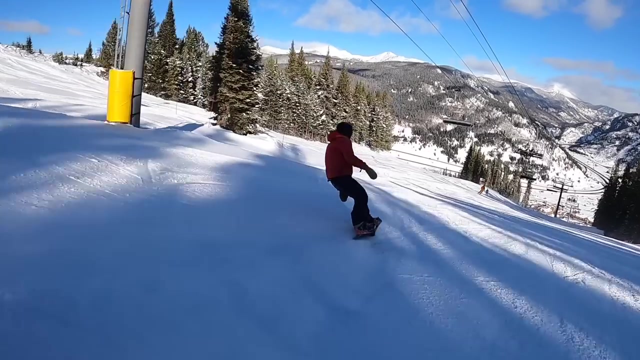 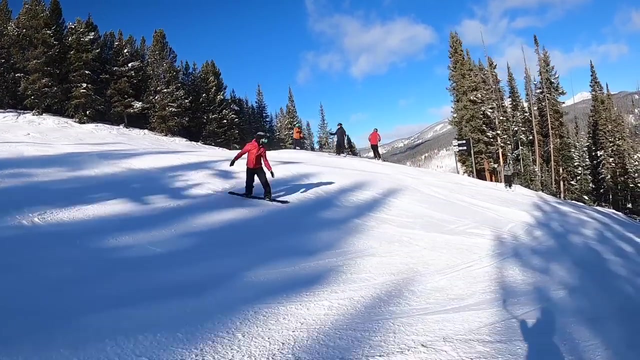 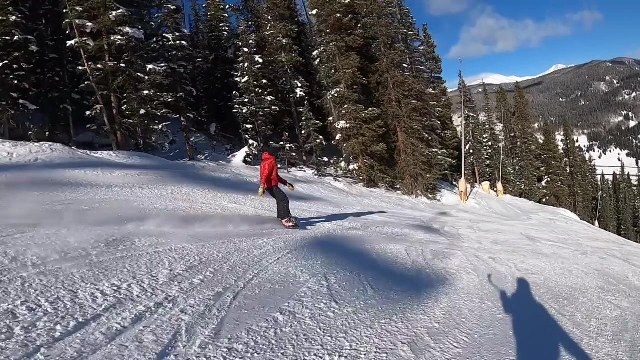 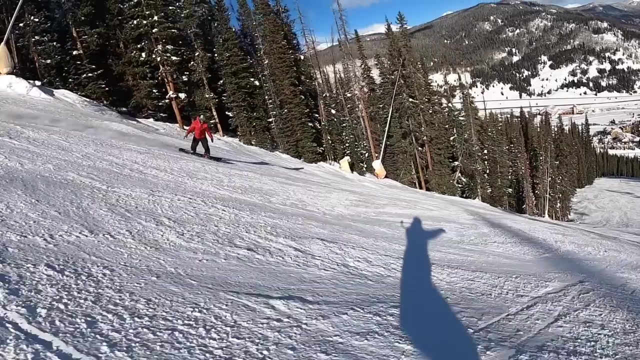 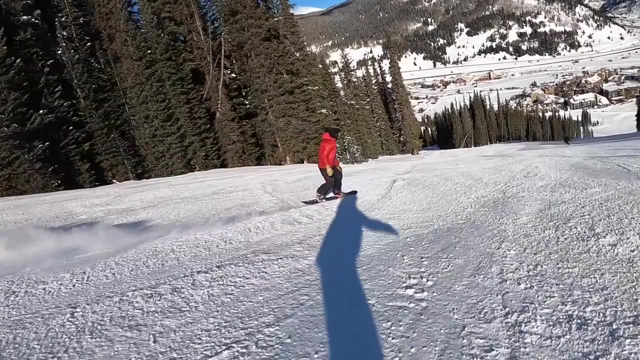 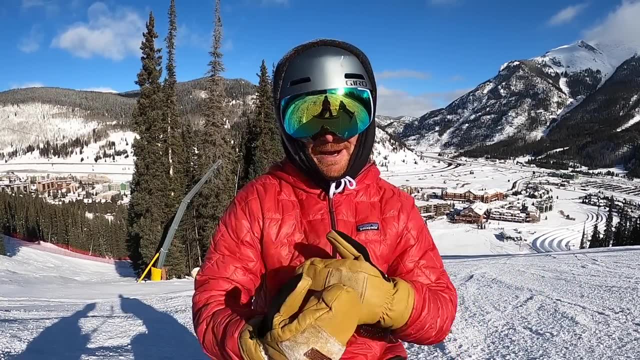 alright, let's get it. Buckhouse. Bye guys. you, Oh, alright guys. so we just went down a super steep run and it was actually a lot of fun. a couple things that I was thinking about as I was ripping up some turns was letting my belly button down the one time live drop, and I was really 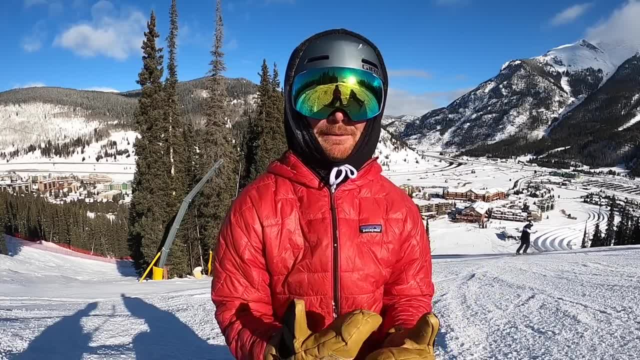 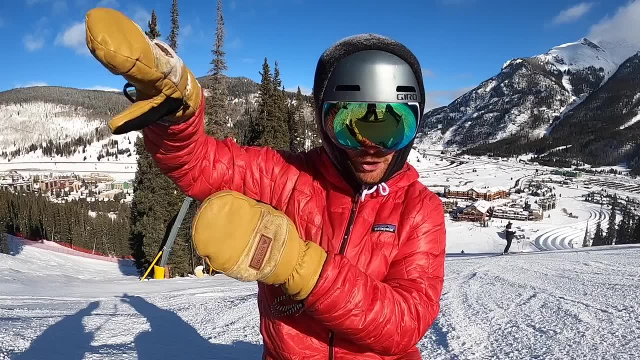 be low and closer to the ground. that made me feel more stable, more in control. the next thing that I was thinking about is I always want to be on an edge, so if I'm able to be on a toe side edge, then I can control my speed at any given time. 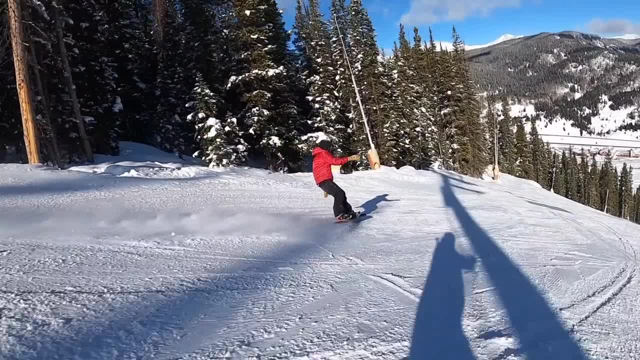 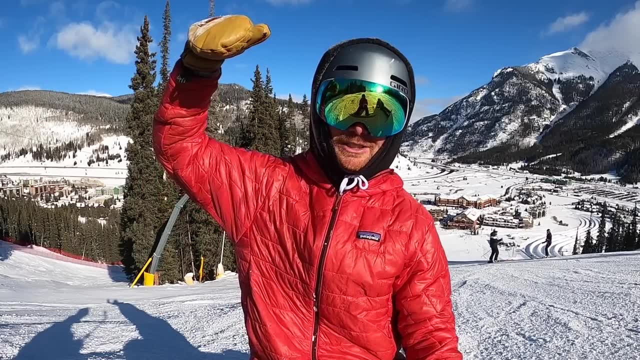 and then I'm on my heel side. I'm controlling my speed. now if I lean back too far I'm gonna have that chatter. so I want to make sure that I understand where my belly button is. obviously you can point your nose of your board straight down the fall line. you're gonna accumulate the most amount of speed. but 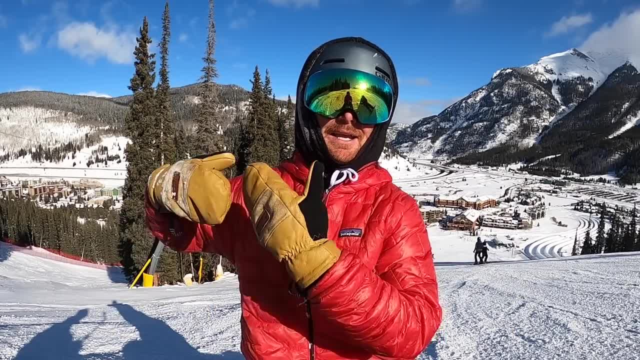 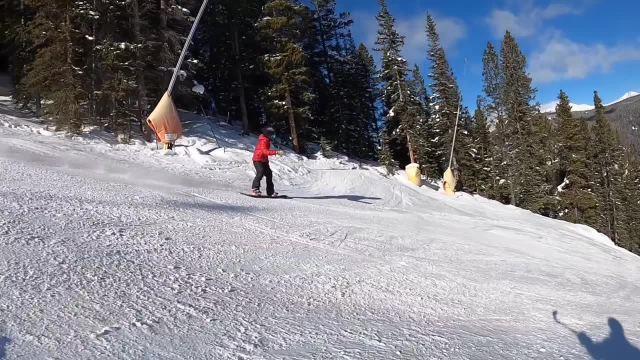 because this video is about being in control. I do want to say and be on an edge so that at any time I can just turn my board across the fall line or I can engage a more of a tilt to slow down. so there's a couple of things that I was. 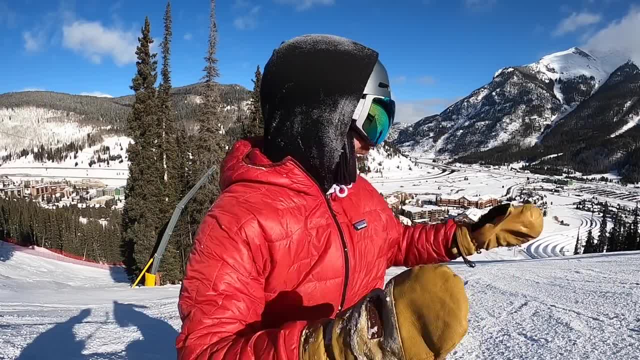 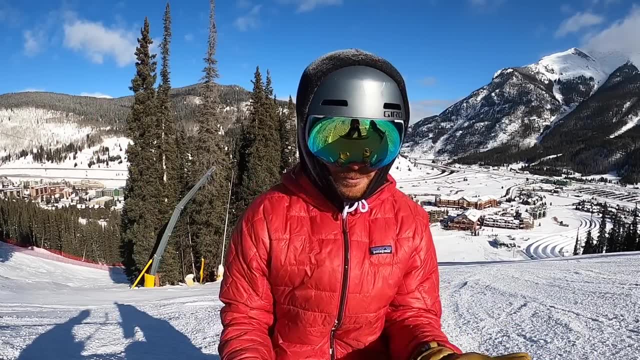 doing on this run. in addition to that, I was keeping my eyes up. I'm looking around as I'm making those turns across the fall line. I'm looking around to make sure that I'm not cutting anyone off. more importantly, I'm not gonna get taken out, because that would suck. I got Jonathan Buckhouse here with a quick tip. 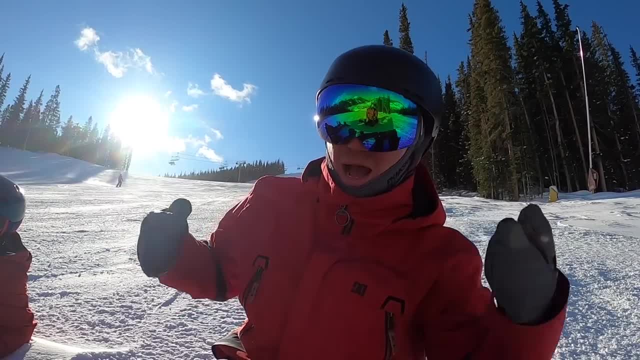 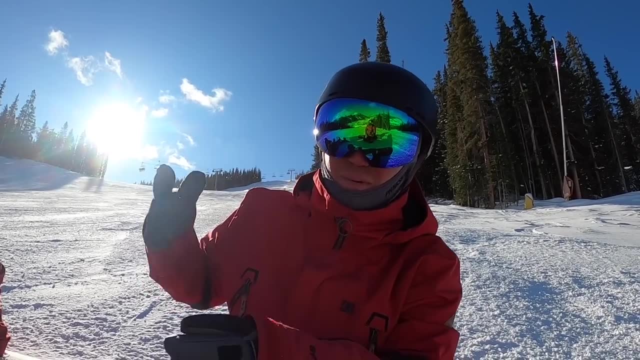 about going fast and being in control. for me, guys, when I am going quick, I'm gonna ride extra fast. I'm gonna actually put my butt to the trip right there, okay, guys. so for me, when I'm going fast and I want- I don't want to bomb a section- I'm 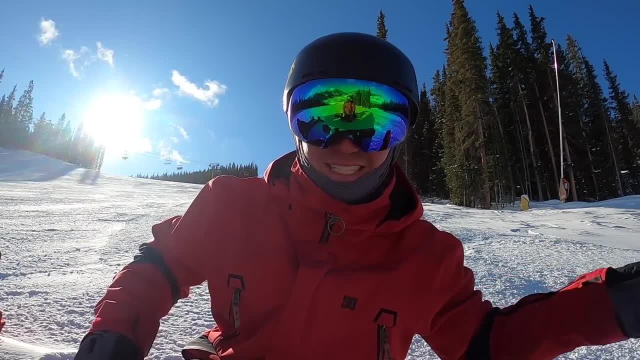 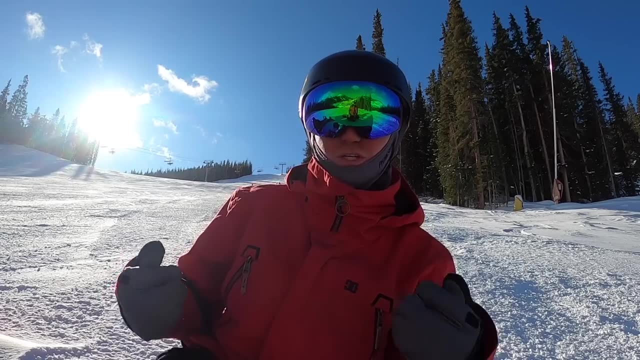 gonna put my butt to the trees that are behind me protecting my blindside. that way I know no one's gonna be coming in and smoking me. so if you are gonna go fast, you can do these small things that are gonna make sure you can go a little. 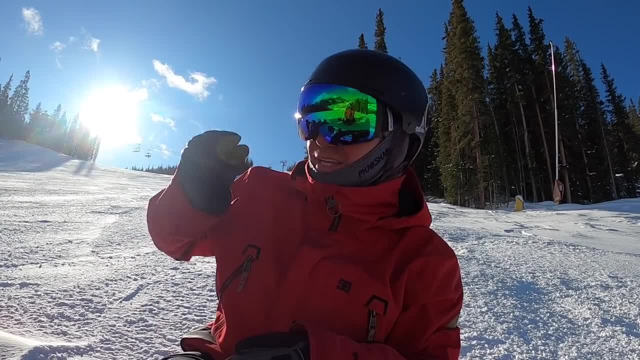 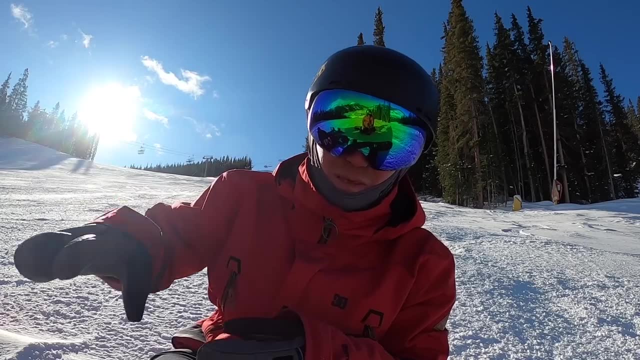 faster but also be extra safe. so if you're a goofy rider, that's gonna be skiers right. if you're gonna be a regular rider, that's gonna be skiers left. I just kind of hug that tree line. I can go a little extra fast, cuz I have to look out for less people, cuz I know the trees are. 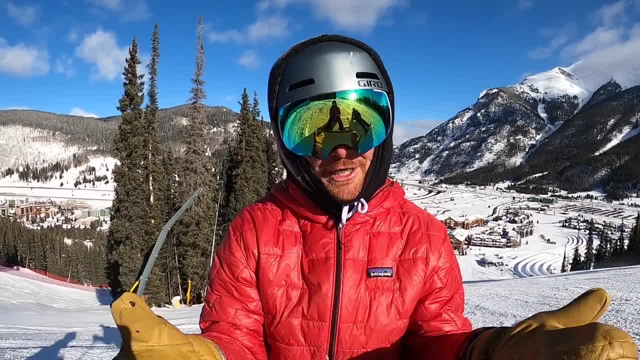 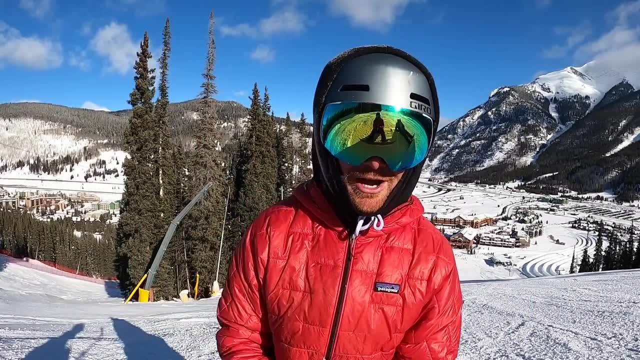 protecting my butt. this whole point in this video is: I know you're gonna go fast, so I want to make sure that you're in control. when it comes to control, I want to make sure that you're able to stop on a dime so that you're not. 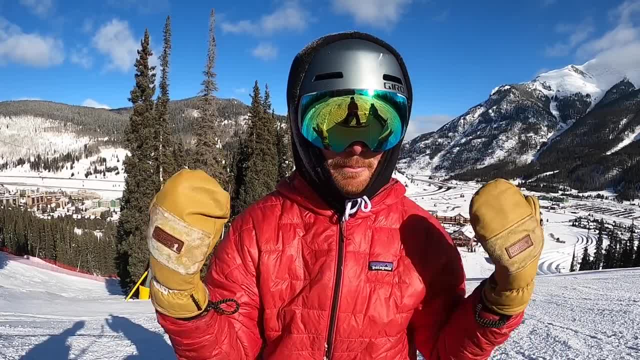 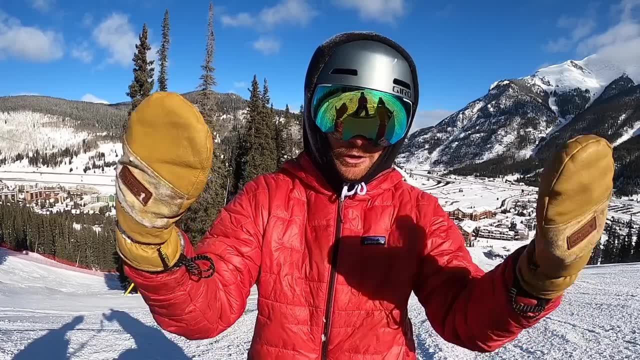 running into a tree, you're not taking someone out and that you're having the best time ever without getting hurt. if you snowboard more, you're simply gonna get better at snowboarding. so this is my way of helping you: snowboard more, getting better and staying healthy. so I hope you enjoyed this video and I'll see you in the next one. 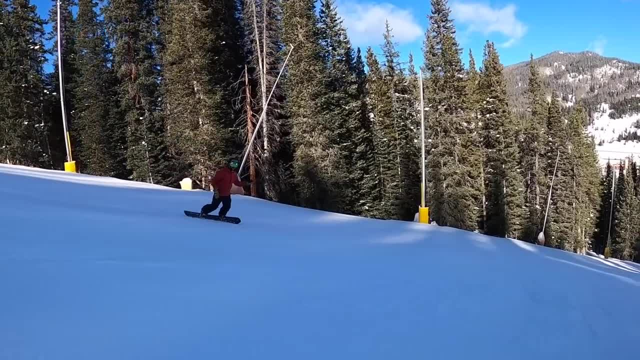 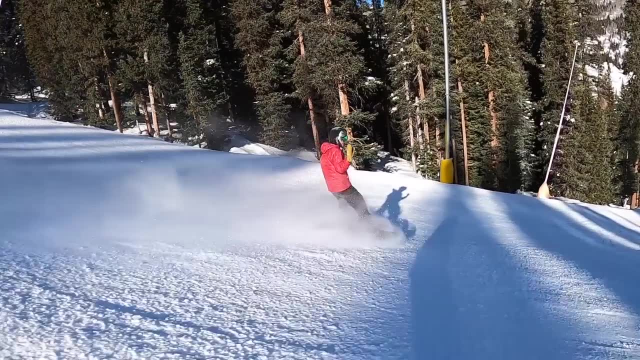 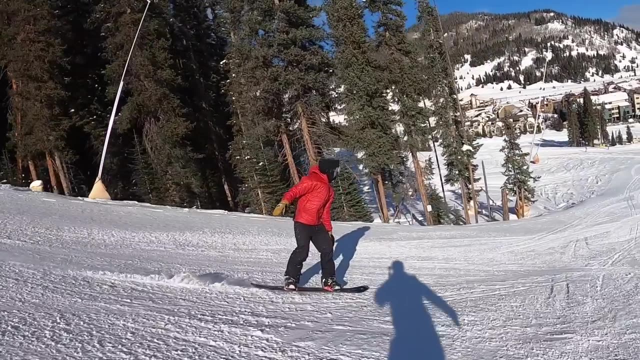 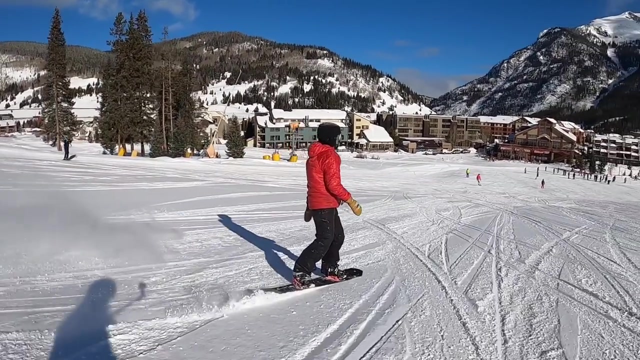 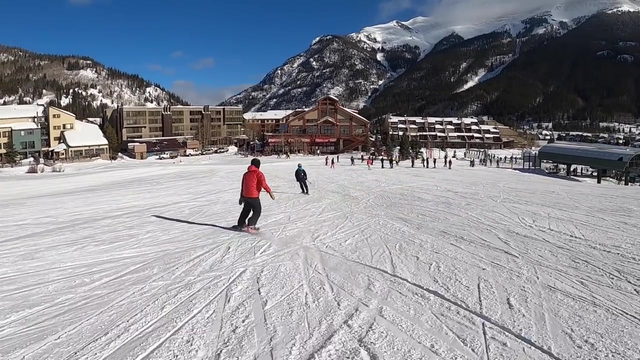 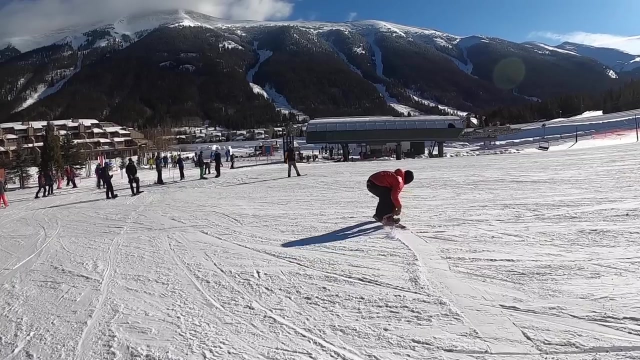 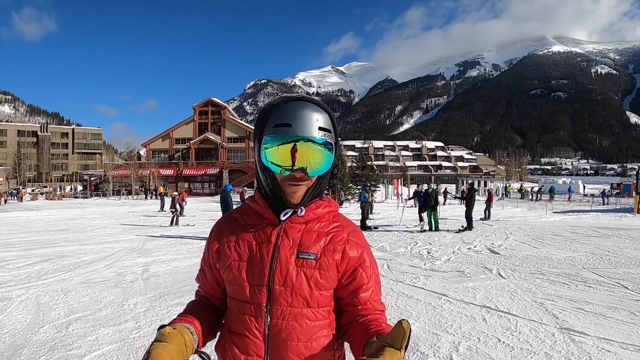 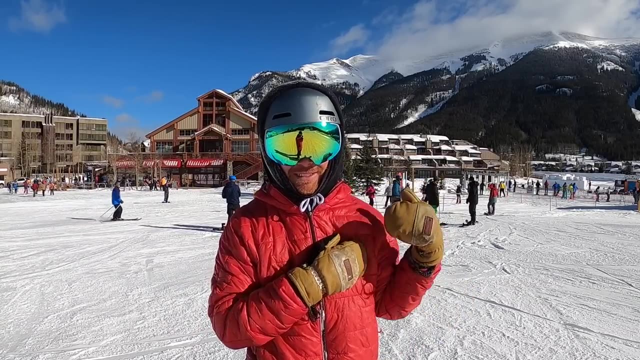 Hope you guys enjoy that. All right guys. so that's my tips for being able to go fast and stay in control. if I miss anything, comment down below and let me know. also, I do have some killing it stickers and some merch that are linked in the description and if